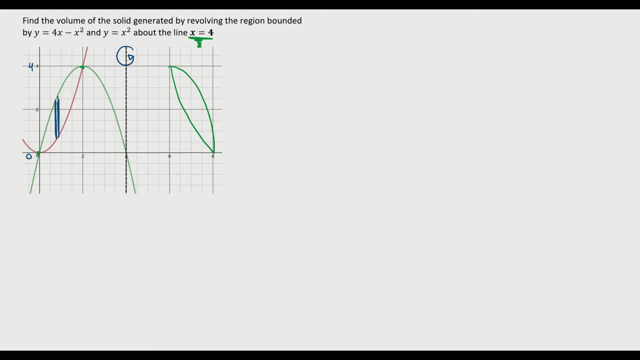 to x. That means my slab needs to be like this and fill up according to the x values. And there, when I now all of a sudden have a slab that is parallel to an axis of rotation, it means we're doing the shell method Okay, and plus you can envision when. 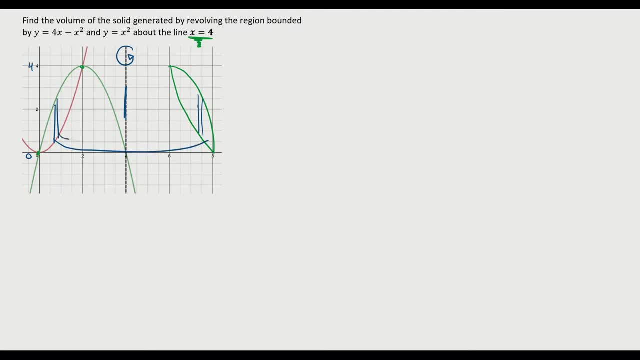 and this really helps, if you can envision this: when this thing swings around, when it swings around that axis of rotation, I all of a sudden have this cylinder idea that pops out. So you see that cylinder and you think shell method. Well, that means when I'm doing the 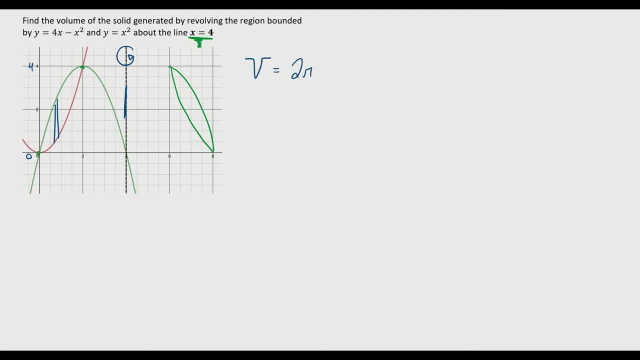 shell method. I know the volume is equal to two pi times the integral from A to B, of the radius times the height times dx, because I'm integrating with respect to y And then I'm going to have a integral with respect to x. But now I need to find my radius, I need to find my height, Both of 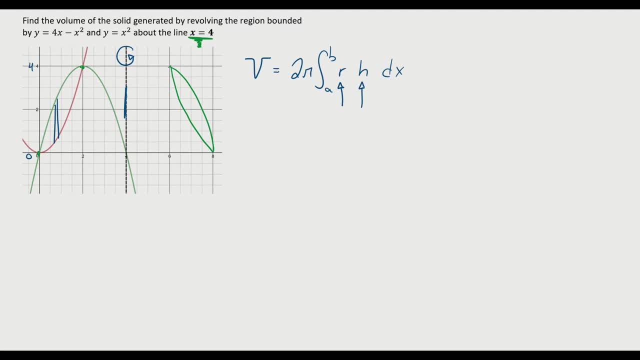 those are functions. okay, a variable, something that's changing. Looking through this, let's break down some of the easy things: the bounds. I am going with respect to x, So it's filling up, So I look from where to where on the x axis I'm going from x equals zero to two. That's where the bounds. 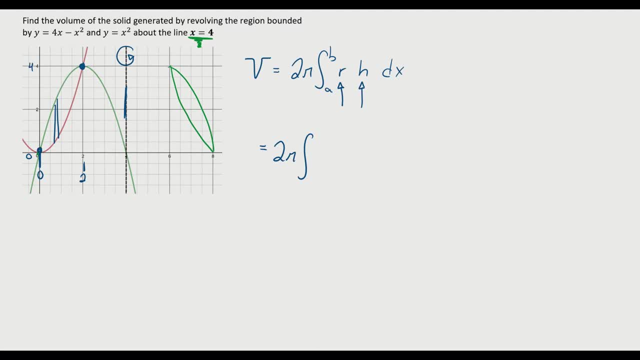 of my region are, And again, I can see that on the graph, But if I didn't have it graphed perfectly here I wouldn't be able to do that. So I'm going to have a integral with respect to x, And then I'm 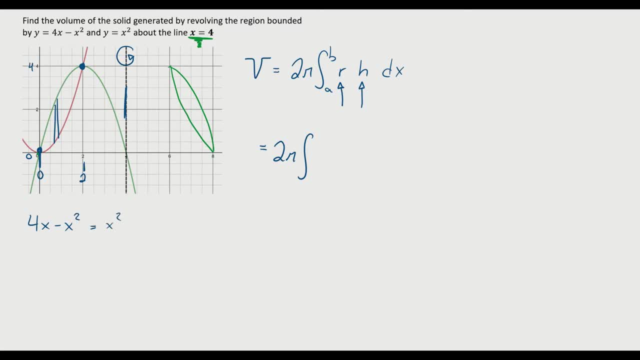 going to have to take the two functions, set them equal to each other and then solve this until you get: x equals zero comma two. So my integral is going from zero to two. All right, what about the radius? the radius of this cylinder? So so one of my shells right there. the radius would be from: 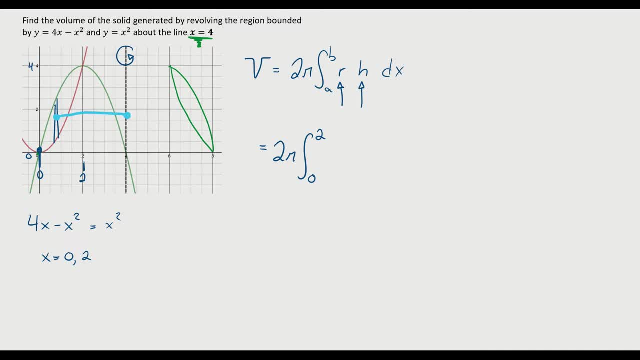 there to here. Now that radius is always. if I'm integrating with respect to x, it might be just x if I'm rotating around the y axis, But if I'm rotating around a different one, such as this time, x equals four. I have to manipulate that a little bit And it's going to end up being four minus x. 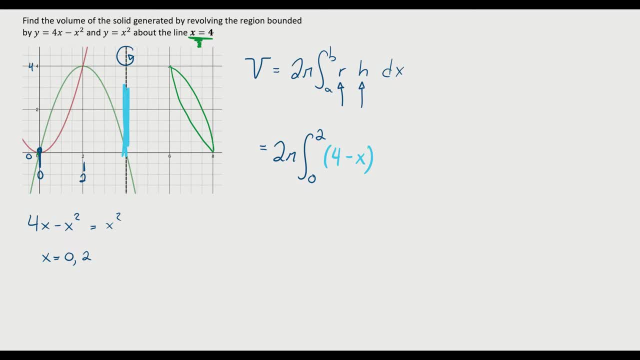 as my radius, Okay. so let's look at one example there. What if I'm right here? my slab is here, Okay, so I have this cylinder. what would be the radius of it? Well, we can see it's three. Okay, the length going from one to four is three. So that kind of makes sense for minus my x. 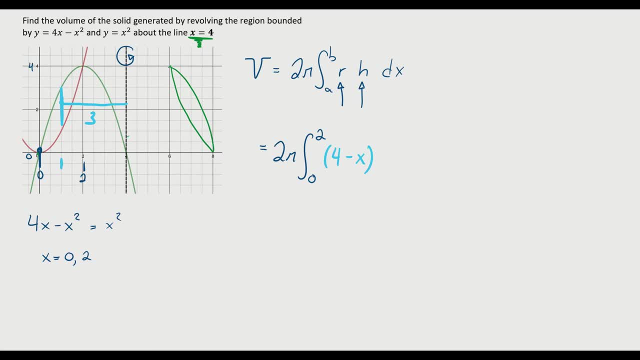 value for minus one. And then what if I'm way up at my top here, that very last shell? Well, in that case, my radius here is two. I'm going from x equals two to x equals four. Once again, that. 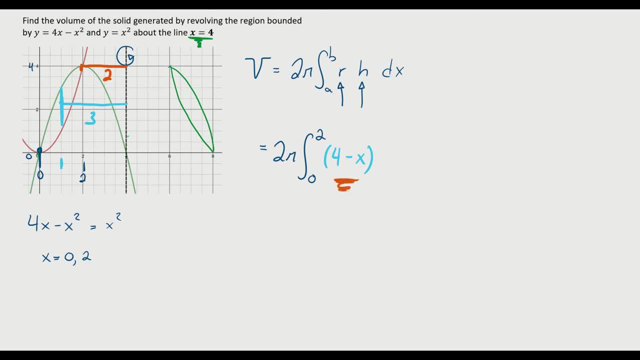 makes sense for minus two. So I'm kind of I'm able to check my radius, thing I put here And it does make sense with a few specific examples. Now, the easy way to do this: whenever you are finding your radius of your shell, you go either top, minus, 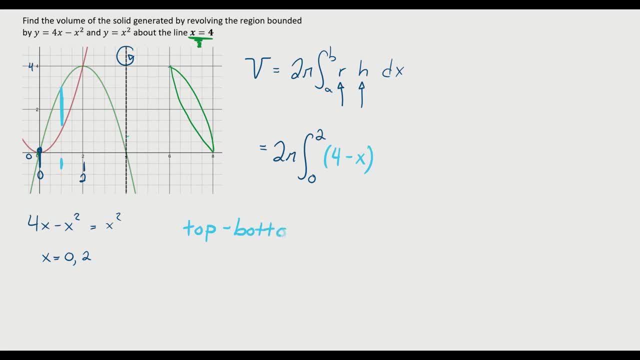 bottom, if you are integrating with respect to y, so going up and down or, like we are in this case, right minus left, And I'm talking about in reference between my axis of rotation and then where my slab is. So see my 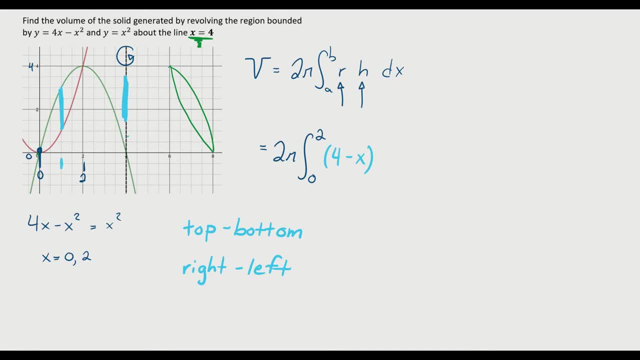 axis is to the right of where the slab is, the original slab on the original region. So you go right minus left, four minus the x. okay, So we get four minus x, then the height, the height of one of these cylinders, one of these shells. it's bouncing between the two curves. So again you go. 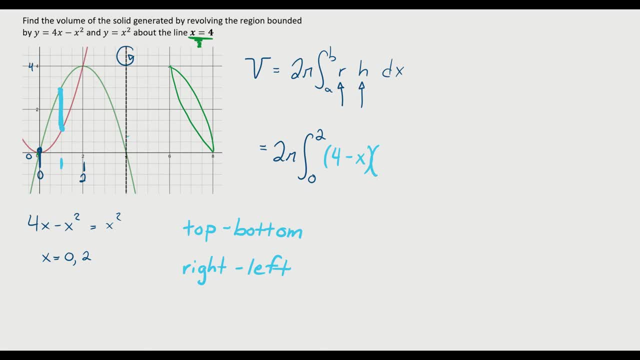 with that idea of top minus bottom or right minus left. this because we got top plus bottom. we're going to go four: x minus x squared, which is my top curve minus my bottom curve of x squared, And then the thickness of each of those shells, dx. Okay, we're going to work through this integral. we've got it all set up So. 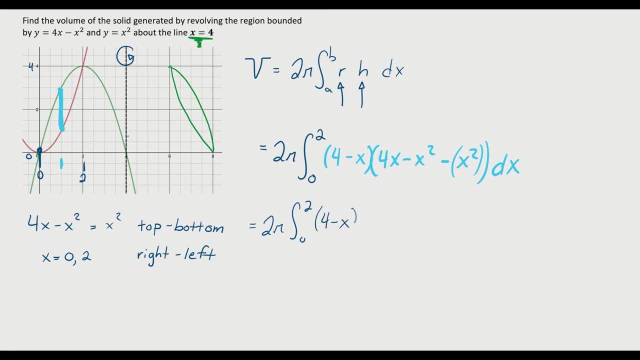 we've done the hard part. Now we're just going to work through it, simplify it a bit before we integrate. Whenever you rotate around that non axis axis of rotation, it adds a little bit to it because, you see, we have to know. 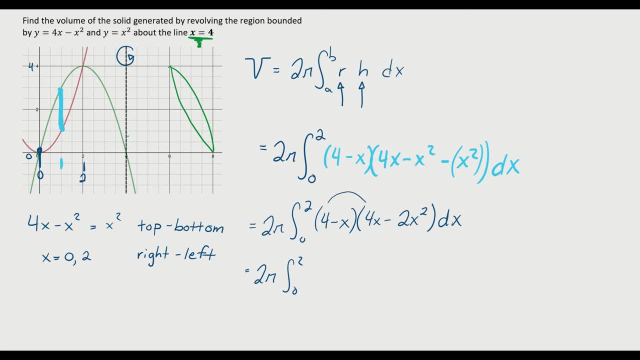 do this foiling with the four minus x. So four times four x is 16 x. four times negative: two x squared. negative eight x squared. you got negative four x squared And then lastly, a positive two x cubed. So I'm going to go through this one more time before integrating combine some like terms. 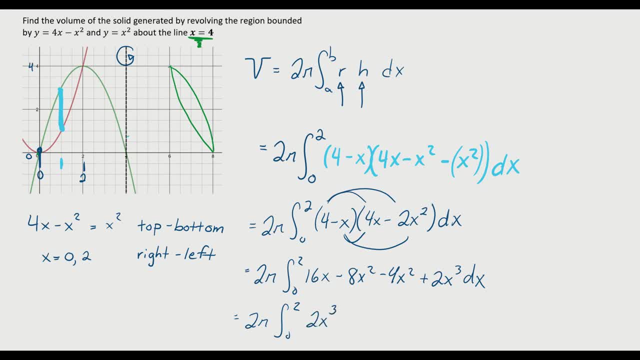 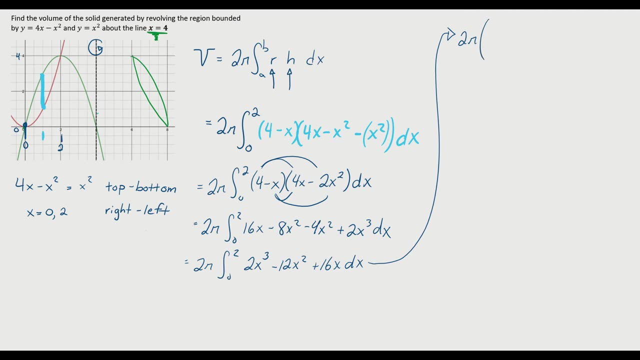 and I'll also put it in standard form, as far as the exponents go: Minus 12 x squared and then plus 16 x. Okay, I'll swing this on up over here and integrate. So we have two pi out front and then power rules. So add one to the exponent and then divide by that, Minus 12 x cubed. 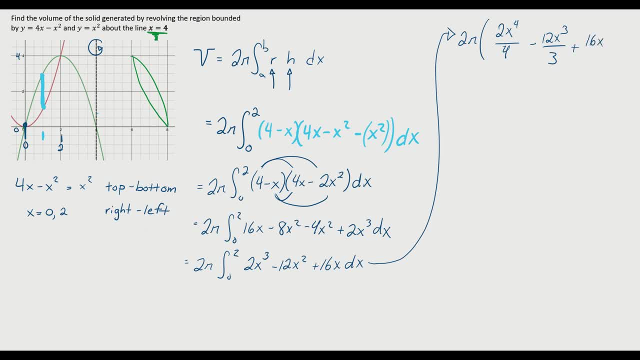 over three, and I'll go through this again and reduce some of these fractions, because they do reduce nicely And we are going from two to zero. Okay, so that equals two pi times x to the fourth. over two minus 12 over three reduces to four x to. 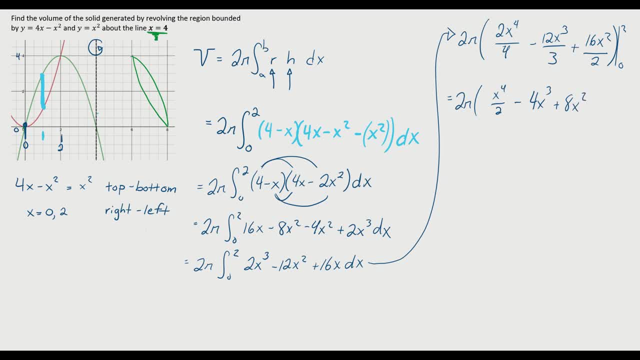 the third plus eight x squared. Alright, so I can adjust to have to evaluate this at two, because when I evaluate at zero it all eliminates. So two to the fourth is 1616 divided by two is eight. Two cubed is eight times four is 32.. 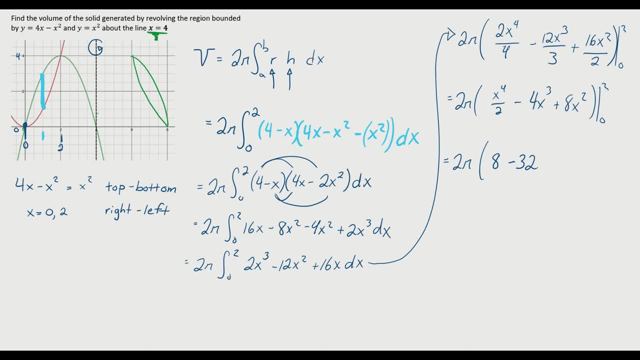 And then two squared is four times eight is 32.. Look at that. I have two pi times eight once the 32s cancel, and then I get 16 pi and we get units cubed. So that is the volume of our solid And that. 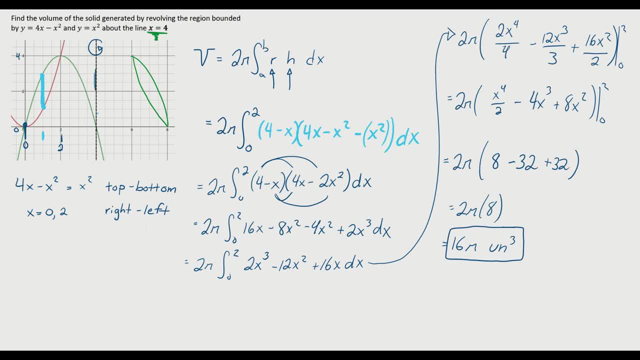 came about by revolving our region around. x equals for a non axis. The big takeaway here two things. When you do your shell method, your slab is parallel to your axis of rotation. That's a shell method Also really helpful. if you can visualize what it looks like when you revolve your slab around your axis, Okay, it kind.